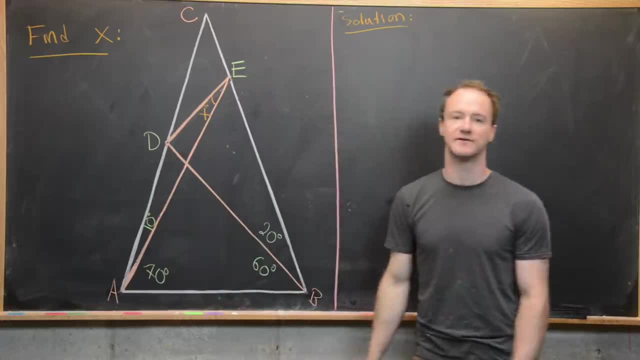 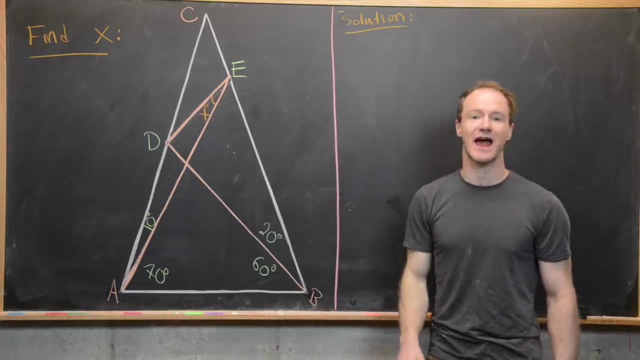 so that we have an angle here of 70 degrees and an angle here of 10 degrees, And then finally we connect D with E and our goal is to find this angle here, X. So let's see what we can get started with. that's pretty easy. 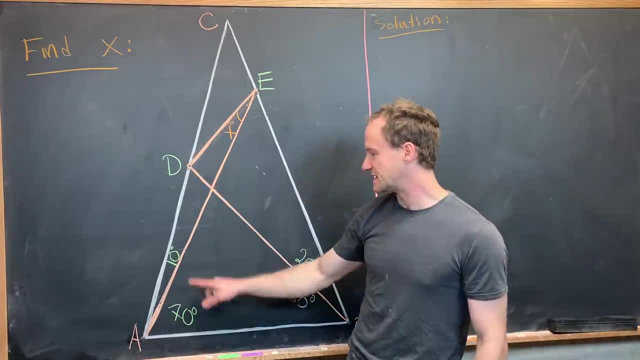 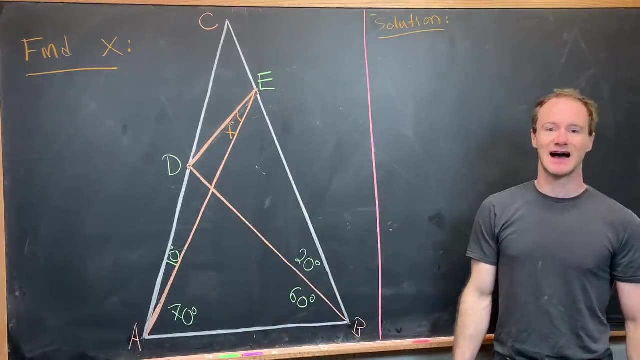 So first we notice that 60 plus 20 is the same thing as 70 plus 10, and so both of these angles right here are 80 degrees, but that's going to make this thing an isosceles triangle, And in 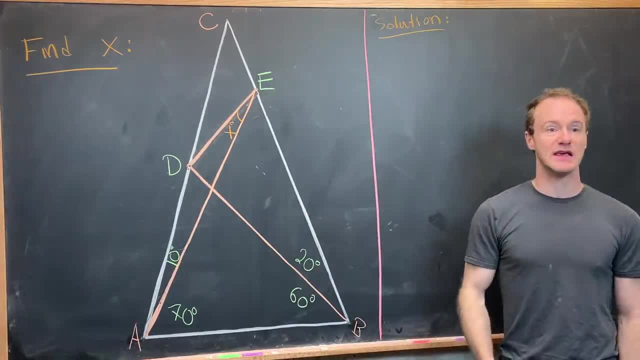 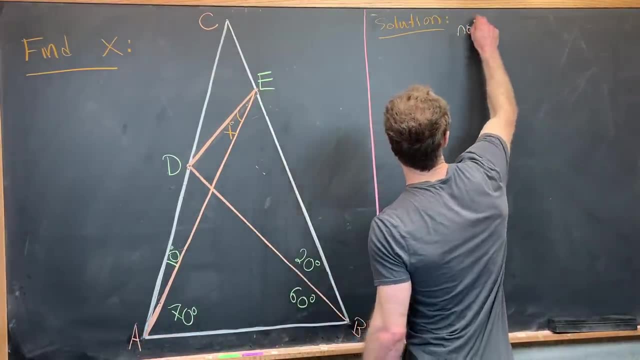 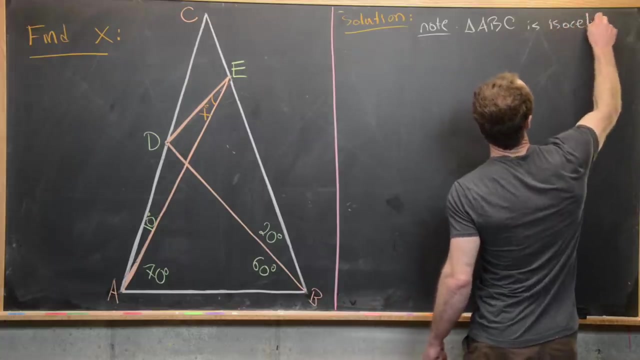 fact, we know that the opposite sides will be equal in length. So in other words, AC is going to be equal to BC. So maybe that's the first thing that we'll notice is that triangle ABC is an isosceles triangle and in fact what we'll use from that is that AC equals BC. 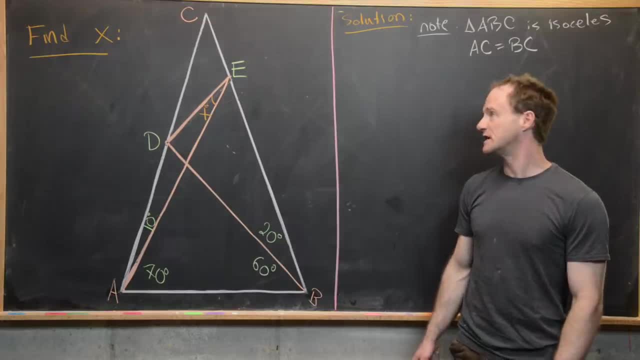 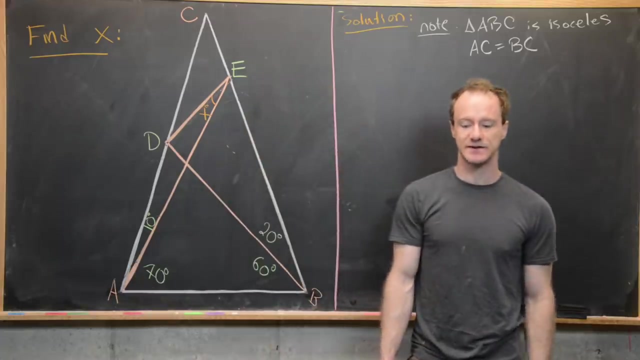 Okay, great. Now the next thing that we can do, which is pretty simple, is fill in some of these angles, and we can do that using the fact that the sum of the angles of a triangle equals 180 degrees. So notice that we know that this is 80, and then this is also 80,, so that adds up to 160,. 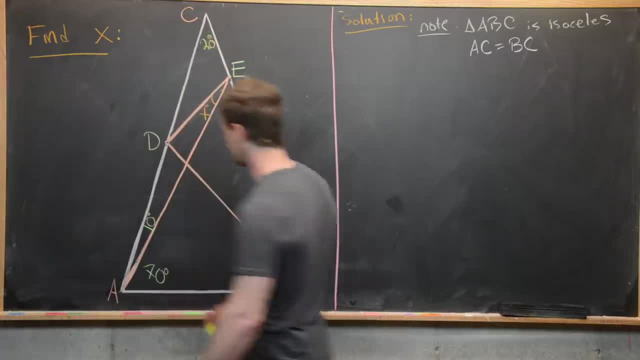 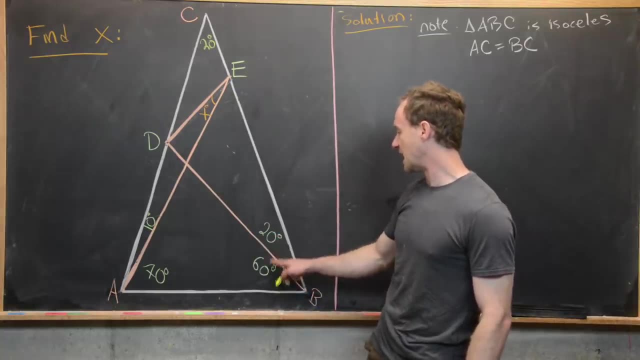 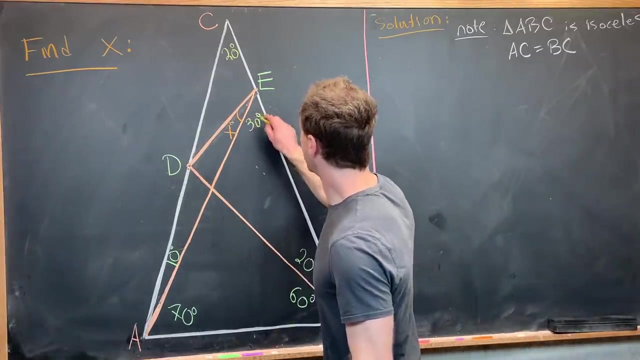 and so that's going to make this angle up here 20 degrees. And now we've also got a triangle here, ABE, and now notice that this is 80, and this is 70, so that totals 150 degrees, which is going to make this angle up here 30 degrees. And then we 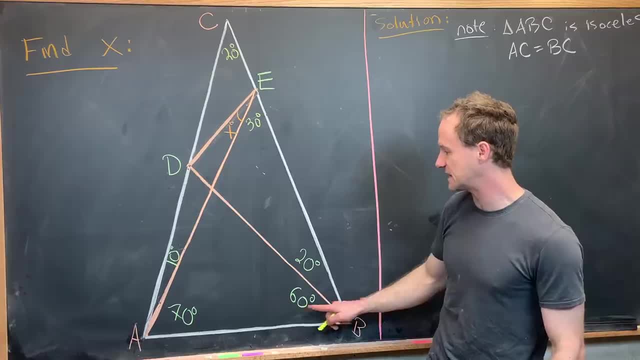 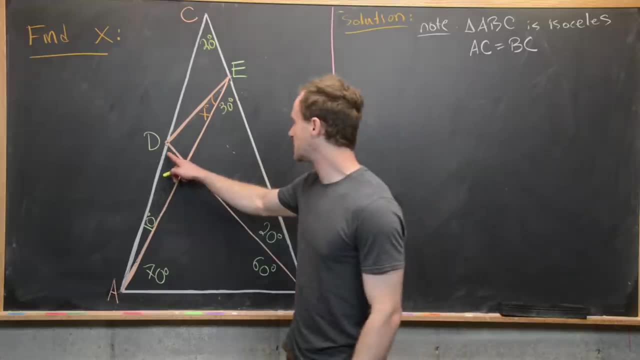 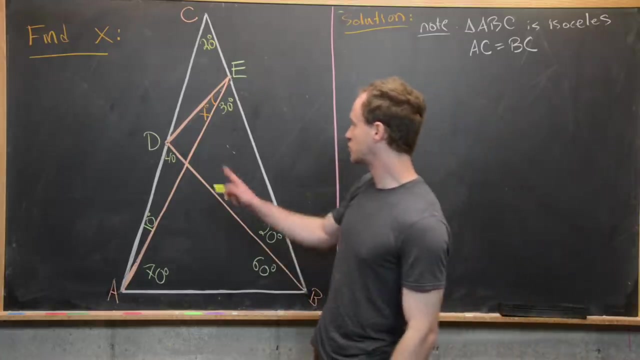 can do something similar over here. So notice, here we've got an angle of 60 and an angle of 80, and so that's going to be a total of 140 degrees, and that makes this angle right here 40 degrees. Okay, and then after that, what we want to do is construct a line going through D, which is: 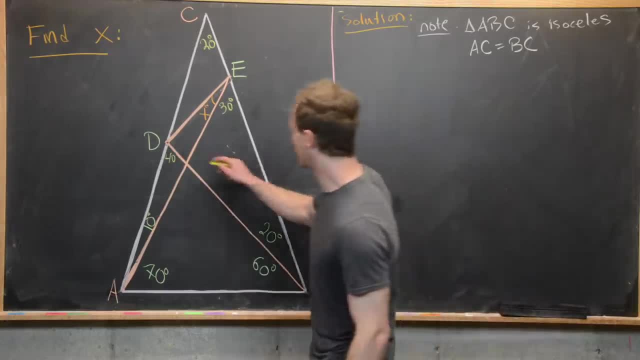 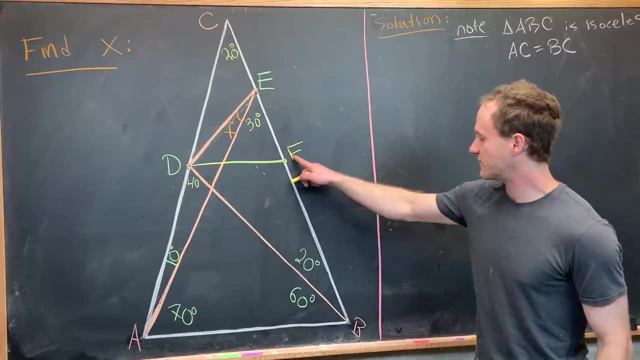 parallel to AB, And so we'll say that other point over here is F, so I'll put a line segment here. We'll call this point here F and we're going to have DF is parallel to AB, So let's maybe go ahead and notice that we're going to construct. 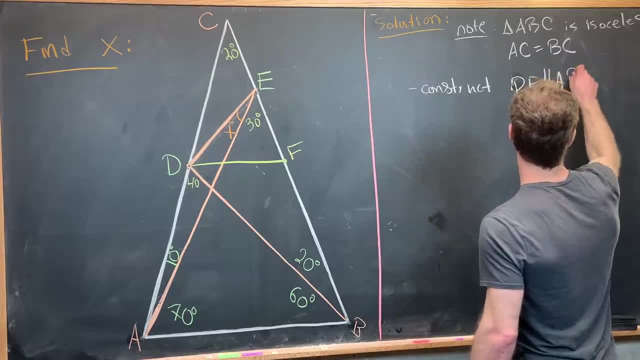 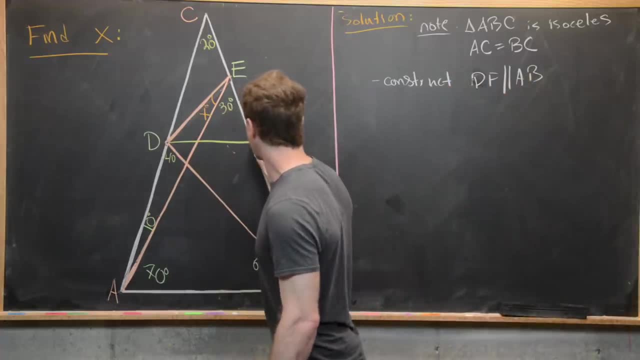 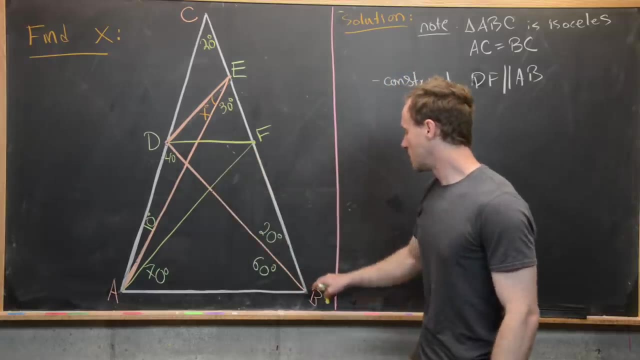 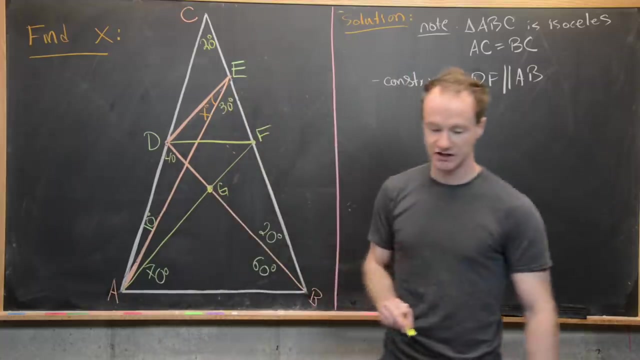 DF, which is parallel to AB. Great, and then from there, what we want to do is connect A with F. so let's do that with a line segment and we'll call the point where AF intersects DB. we'll call this point G. So we've got a point here which we've created, G. and then, finally, we want to construct one more. 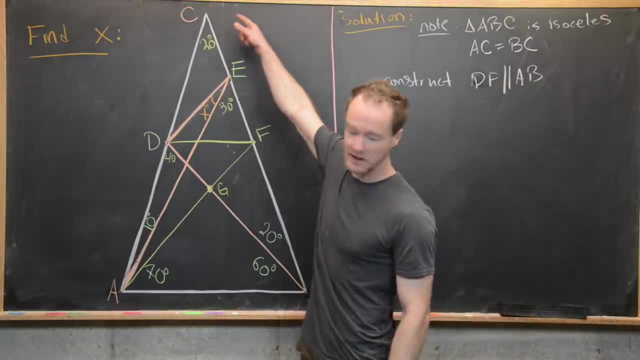 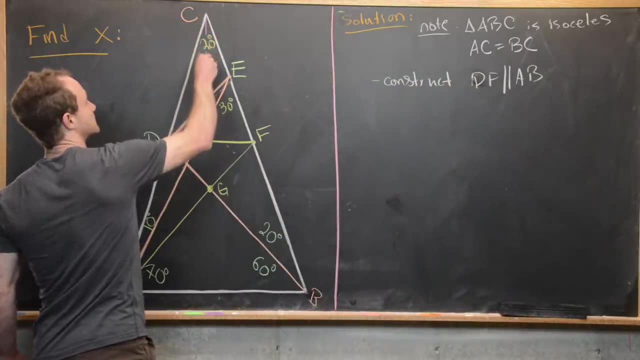 line segment and that will be the line segment up here from C, down here to G. So let's go ahead and do that. So we've got this line segment here, C to G. So that's going to be another important line segment to consider. 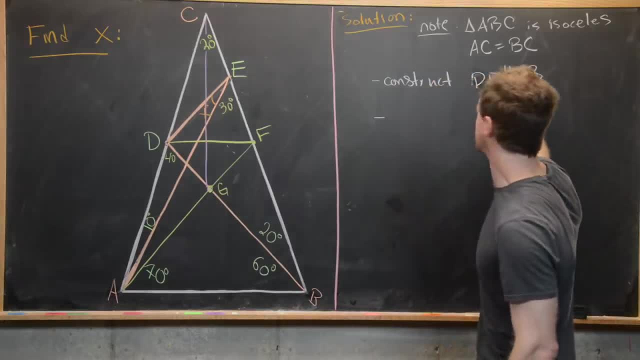 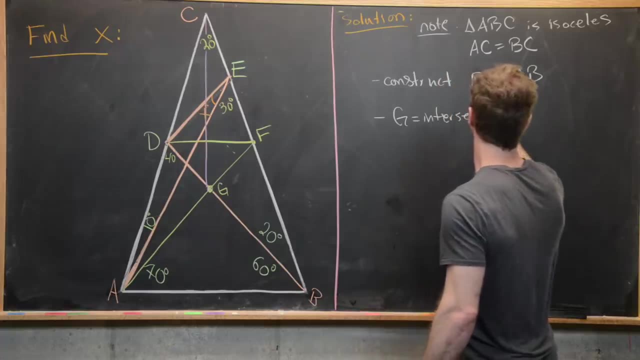 Okay, so let's point out what we did over here. So we constructed DF, which is parallel to AB. We took G to be equal to the intersection of AF with BD. That's one thing that we did. and then we took G to be equal to the intersection of AF with BD. That's one thing that we did. and then we took G to be equal to the intersection of AF with BD. 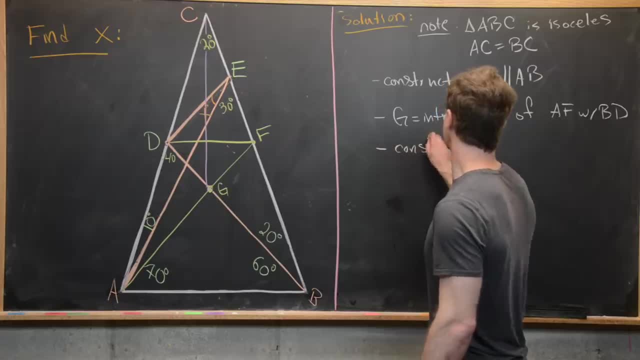 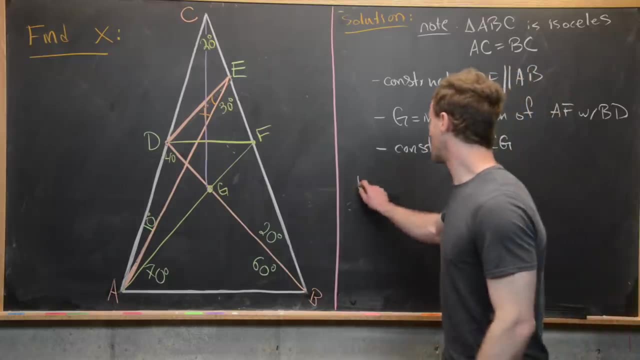 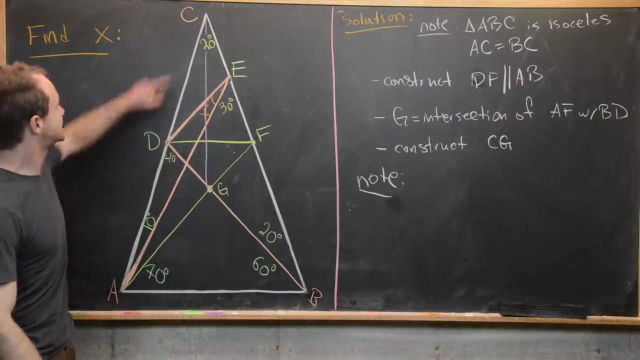 That's one thing that we did, and then we also constructed CG, that line segment. Okay, so the next thing that we want to do is notice that we have the following: So this triangle up here, CDF, is similar to the triangle CAB, and so that's pretty clear, because 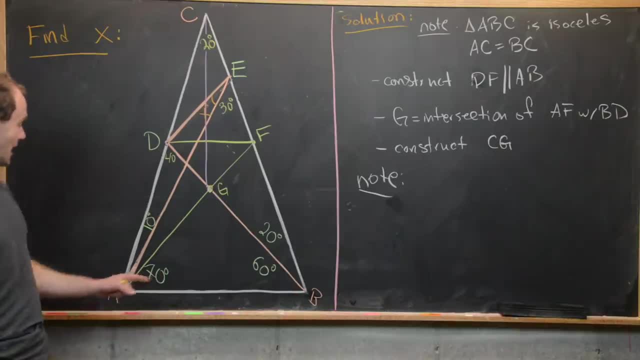 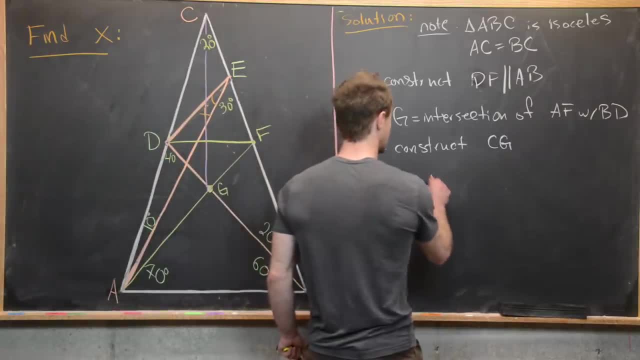 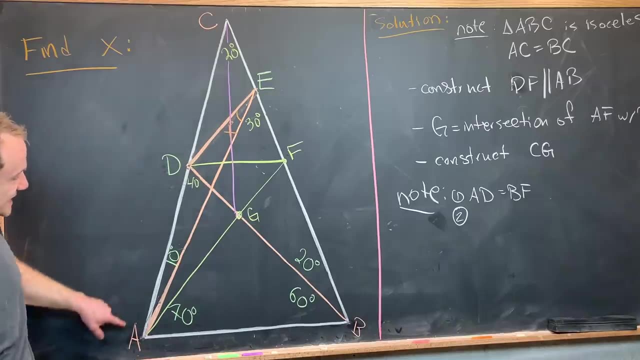 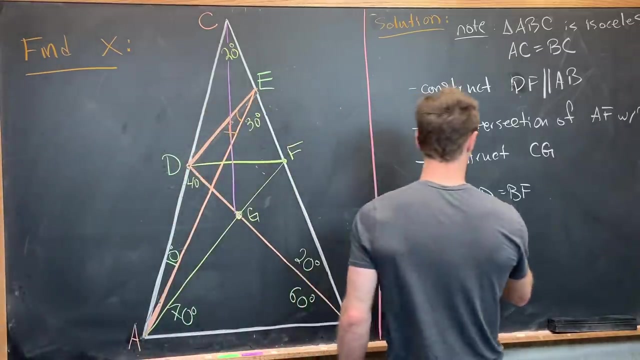 And γ is congruent to this line segment here, BF. so that's one thing that we want to notice. AD is congruent to BF- Great. and another thing to notice is that angle DAB is the same thing as angle ABF. Those are both 80 degrees, So let's write that down. So angle DAB. 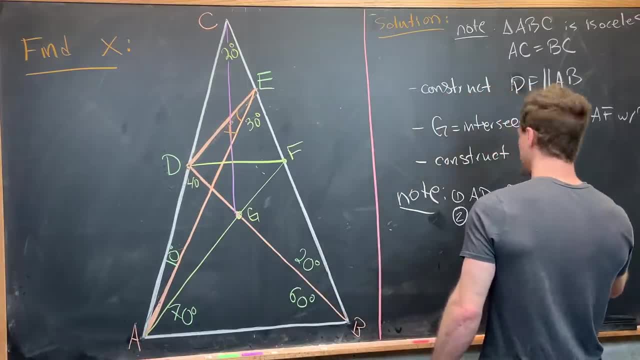 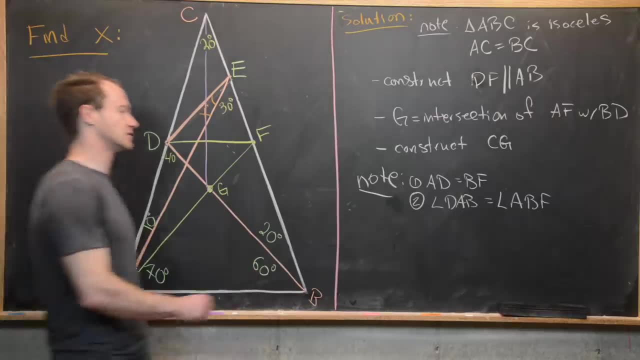 is equal to angle ABF. And then finally, something that's pretty trivial, which is line segment A. B is equal to the angle J, B. and then finally, Lee circle, which is pretty trivial, which is line segment A, B. AB is congruent to itself. So here we have line segment AB is congruent to: 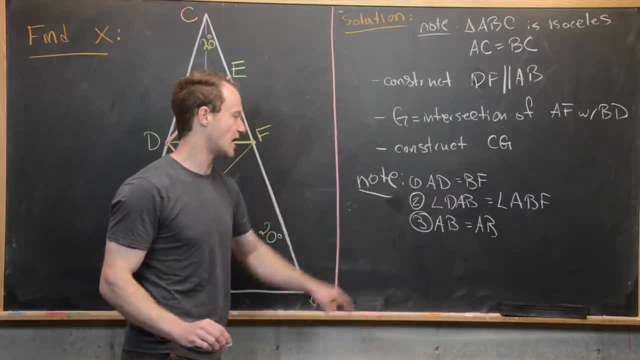 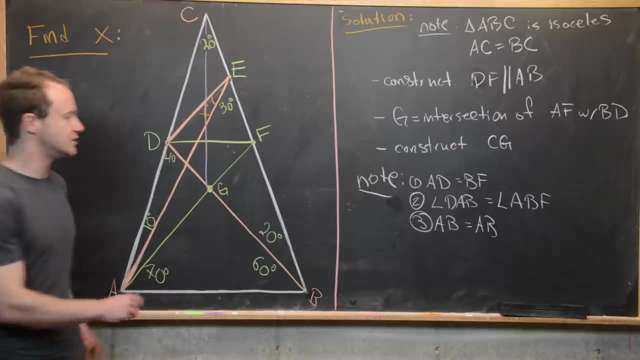 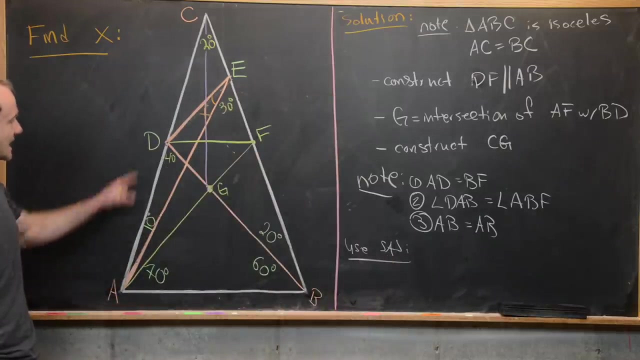 itself. And so now notice, we've got two triangles which have sides that are congruent and angles which are congruent. So we can use the side angle side theorem, So use SAS. So that's going to tell us that triangle ADB and triangle AFB. 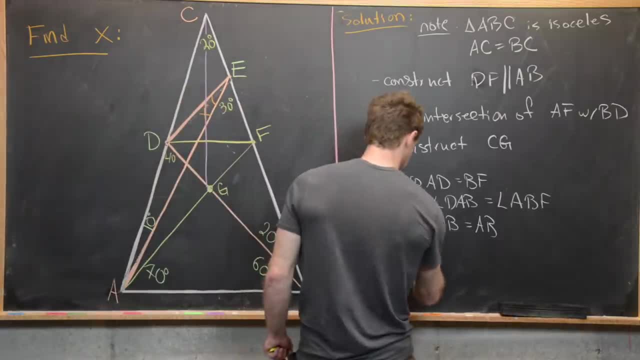 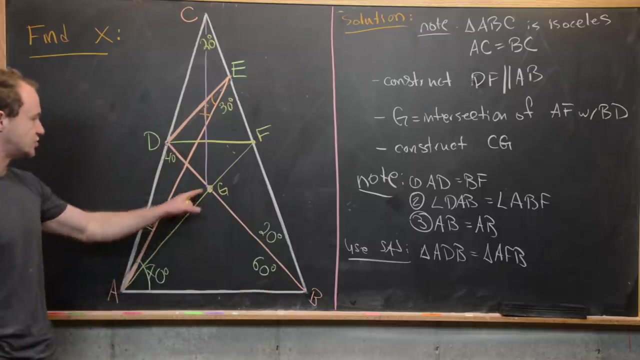 are congruent, So great. So let's go ahead and write that down. So triangle ADB is congruent to triangle AFB. Okay, good. So now we can use this congruence of triangles to calculate angle BAG. So it looks like in the picture that this is. 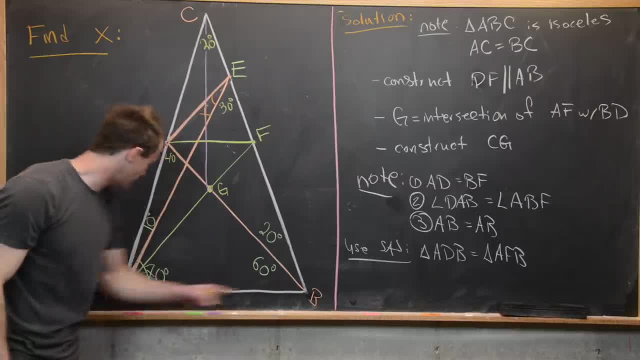 70 degrees, but recall that 70 degrees is angle BAE. So notice, angle BAG will be equal to angle BAE. So now we can use this congruence of triangles to calculate angle BAG. So it looks like in the picture that this is 70 degrees, but recall that. 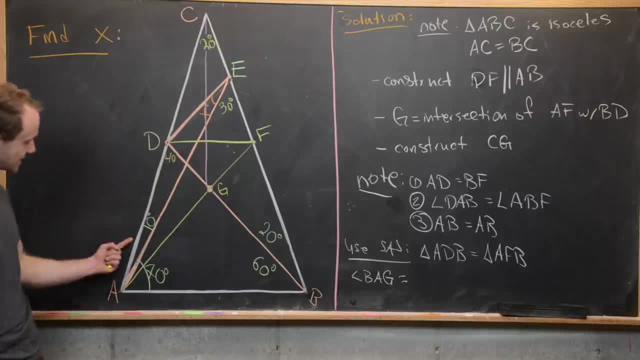 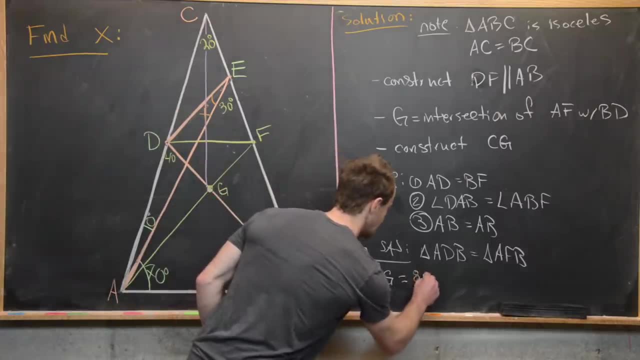 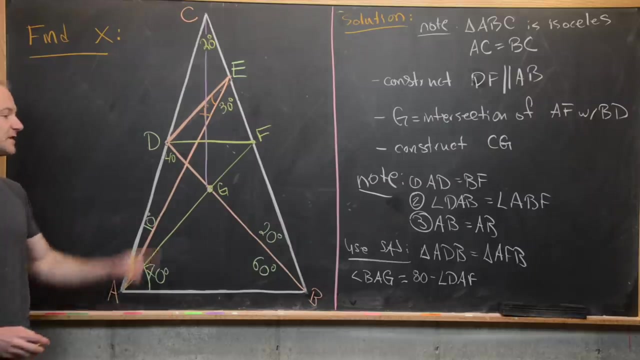 angle BAE will be equal to angle DAF. So this angle is 80 minus the angle DAF, And that's clear, because this entire angle is 80 degrees And what we're doing is taking away this part. So here we have: this is 80 minus angle DAF. Okay, good, But then we know. 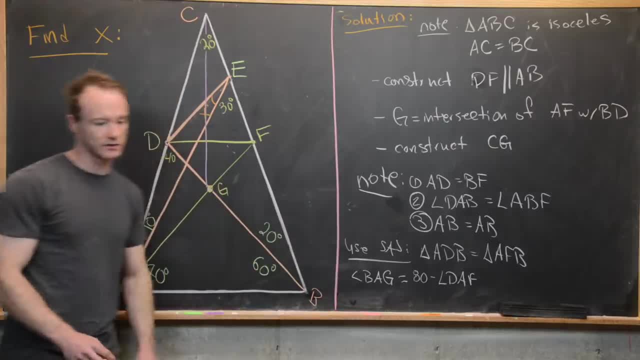 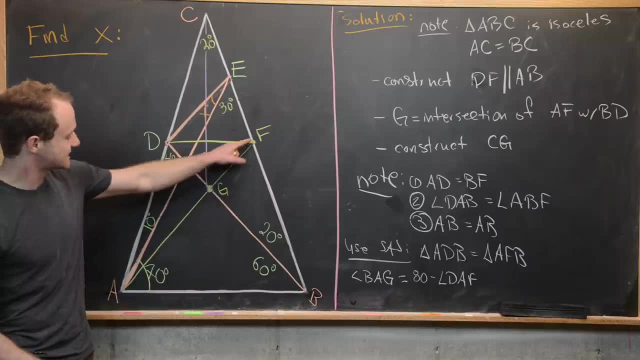 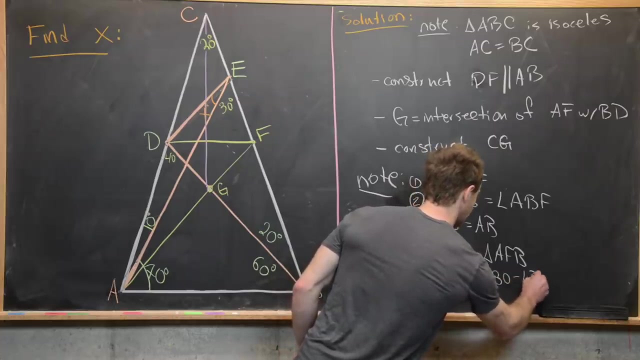 something about angle DAF because of the congruence of these triangles. We know that that is congruent to angle FBG. So let's look at this FBG So we can just write that down. So this is 80 minus angle FBG, But it's given that angle FBG. 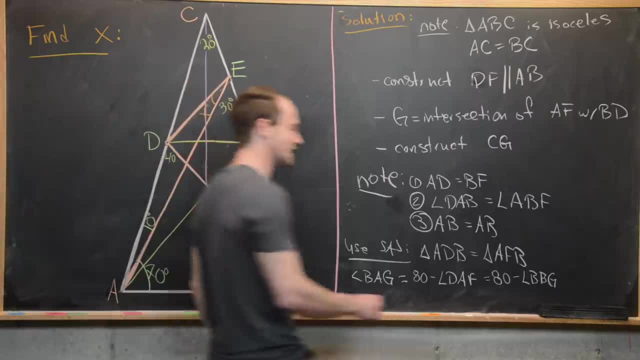 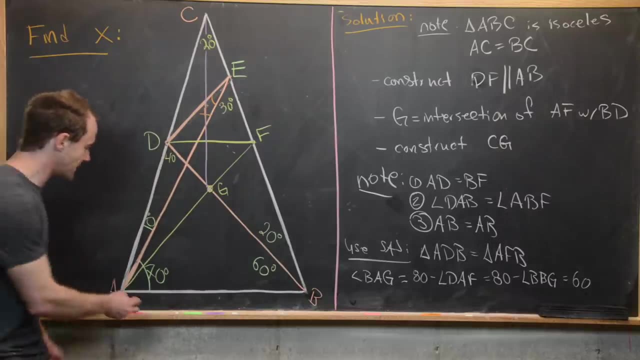 is 20 degrees, So we have that. this is 80 minus 20 or 60 degrees, So we've got angle BAG is 60 degrees, So let's maybe add that in here. So this whole thing is 70 degrees, which makes this little. 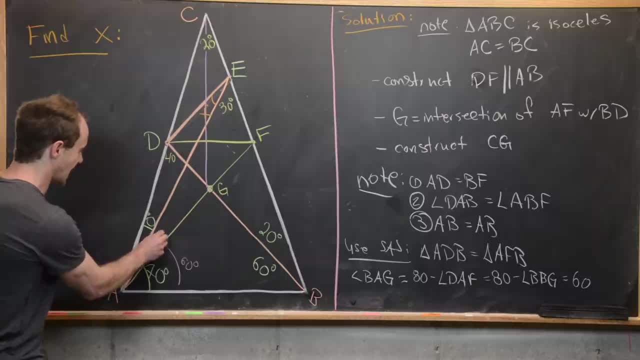 thing here 60 degrees, which makes this thing here 10 degrees. Great. So now we've partitioned this entire 80 degrees into 60 plus 10 plus 10.. Okay, great, So I'm going to go ahead and erase. 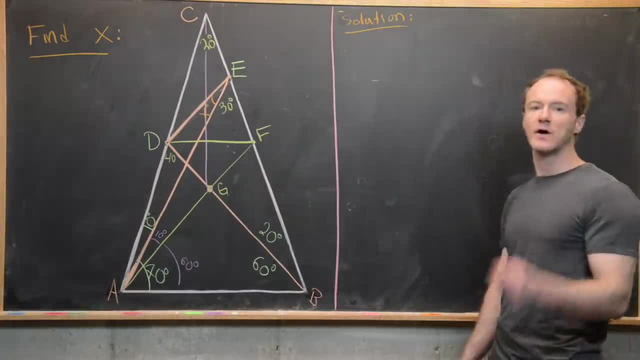 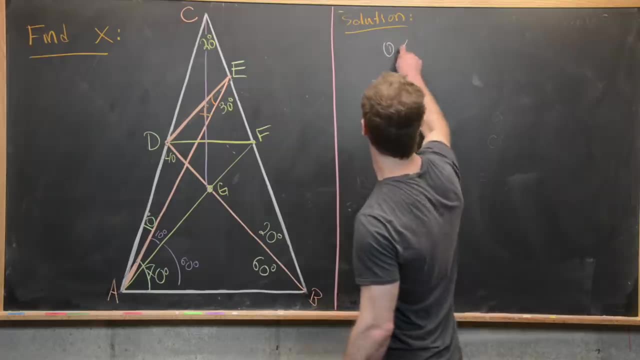 that part of the board, and then we'll get on to the next step. Okay, so now we're going to construct another set of similar triangles, And we can do that in the following way. So first of all, we'll notice that angle CAG C-A-G. 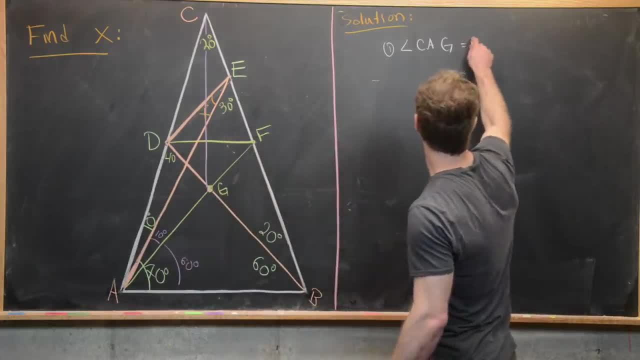 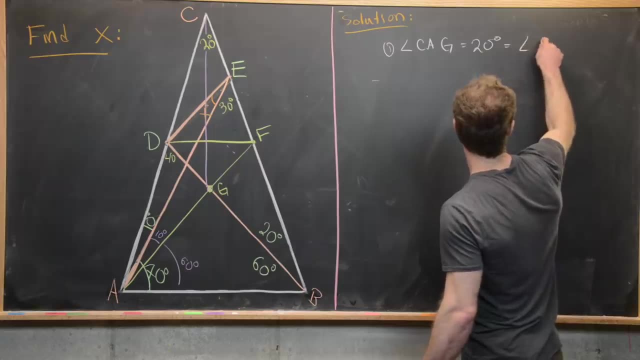 So that's 10 plus 10 degrees, So that's equal to 20 degrees, But that's the same thing as angle CBG. So here we have: this is angle CBG, Okay, good. And then another thing that we know. 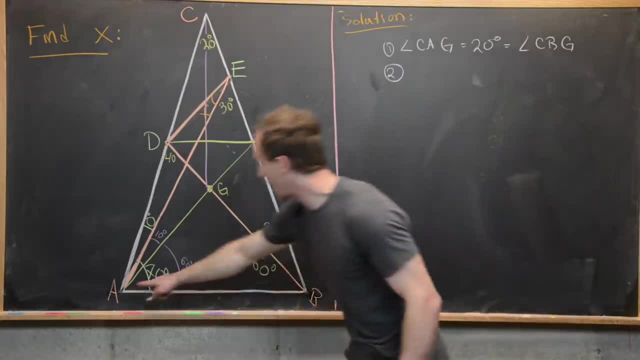 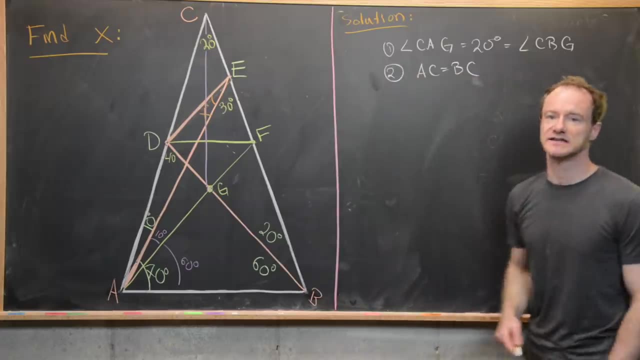 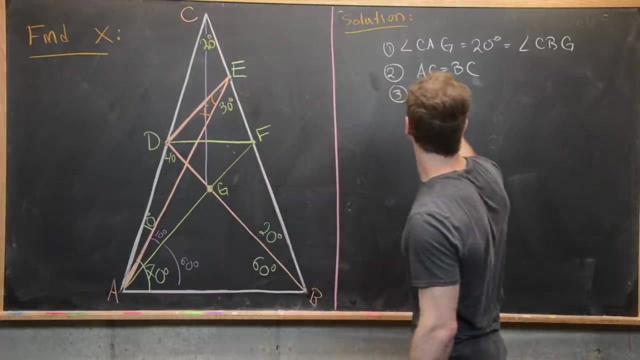 which is kind of from an earlier calculation, is that AC is equal to BC, And that's because the big triangle is isosceles. And then, finally, we can have this trivial fact which is CG is equal to itself, And so that's going to give us by SAS again. 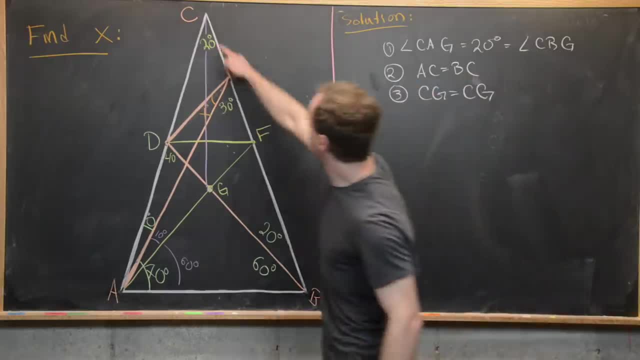 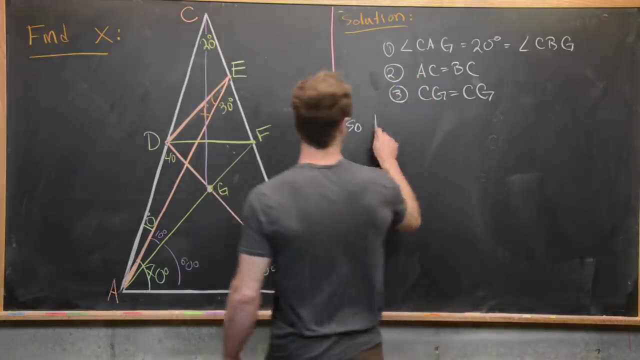 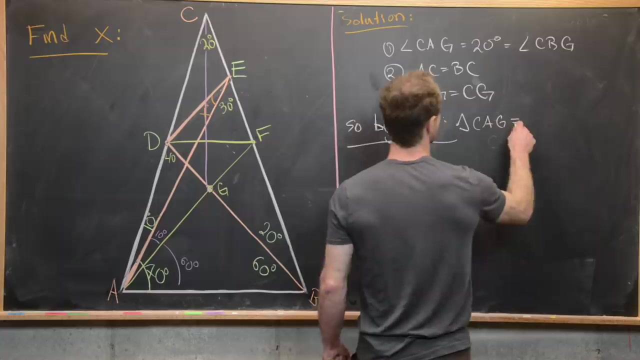 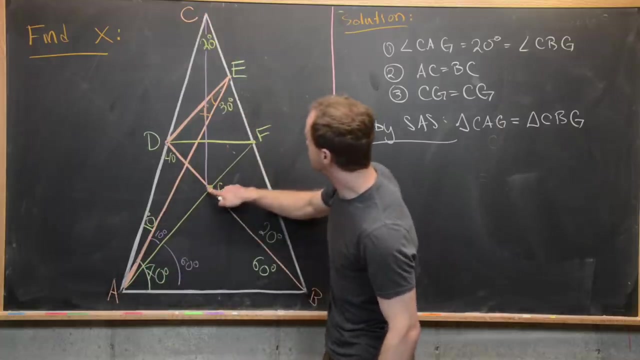 the congruence of two more triangles. So we have triangle CBG is congruent to single triangle CAG. So by SAS, like I said, triangle CAG is congruent to triangle CBG. So let's see what we have: CAG. 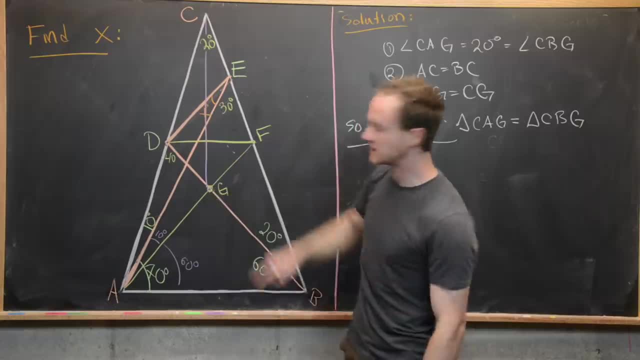 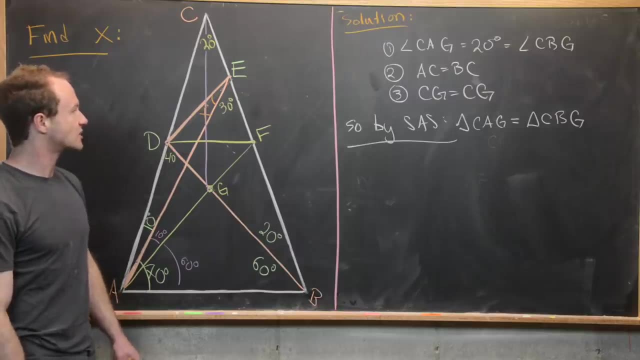 so this triangle right here, and then CBG, so that triangle right there. Okay, great. So now what we want to do is use the fact that these triangles are congruent to notice that that means that angle ACB is congruent to triangle CBG. So that's going to give us by SAS, like I said. 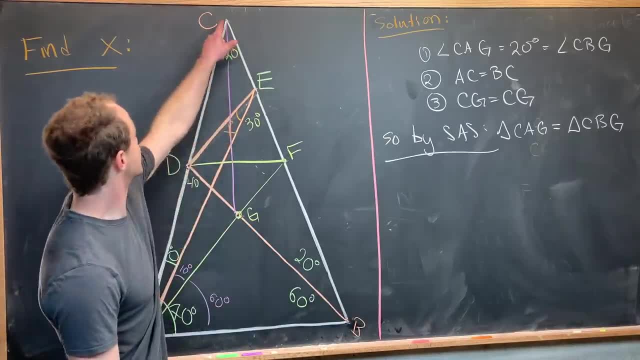 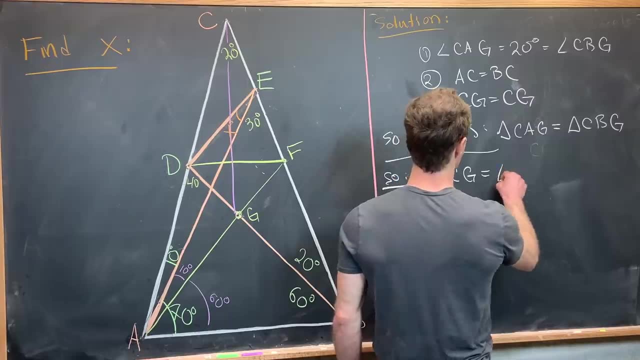 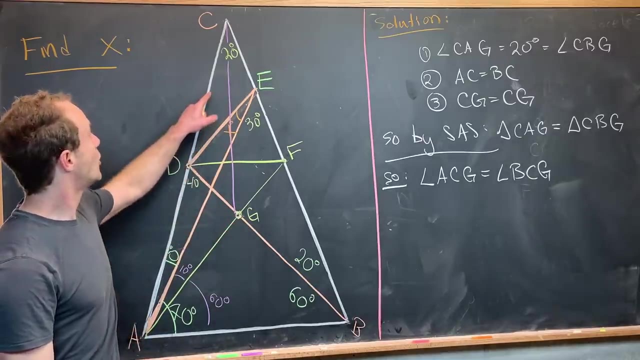 angle ACG is congruent to angle BCG, So let's go ahead and write that down. So angle ACG is equal to angle BCG. So that's new from the congruence of the triangles. Good, But we notice that those 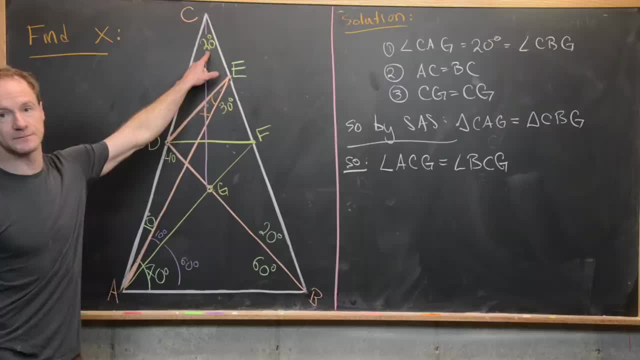 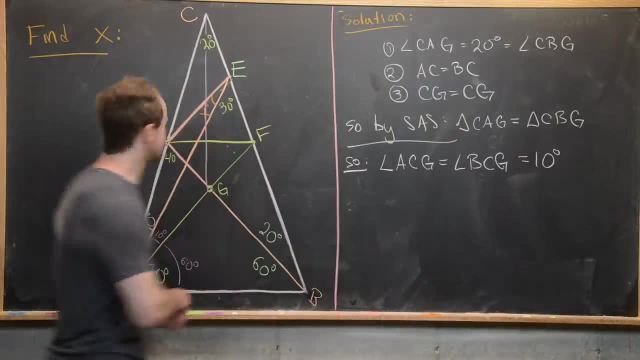 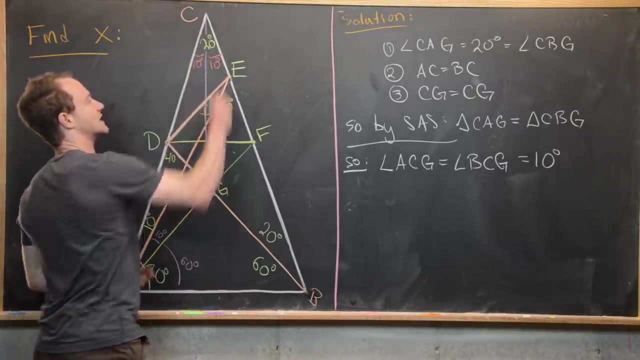 two angles sum to 20 degrees. But if those two angles sum to 20 degrees, then each one is equal to 10 degrees. So let's maybe add that to the triangle. So let's go ahead and write that down, Add that in there. So here we have. this angle, right here is 10 degrees, This angle right here. 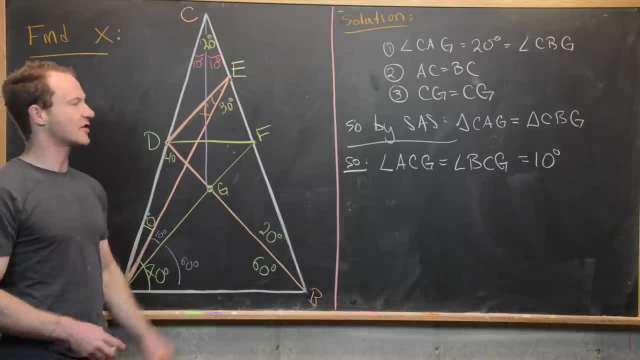 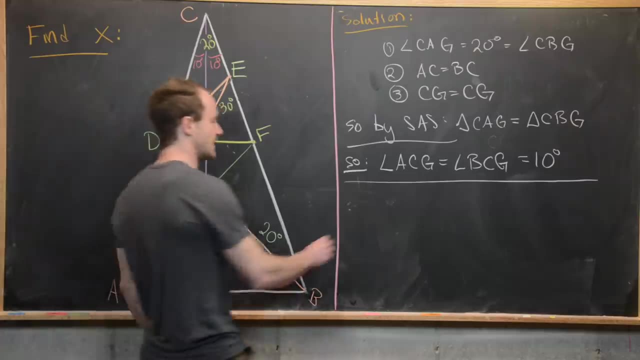 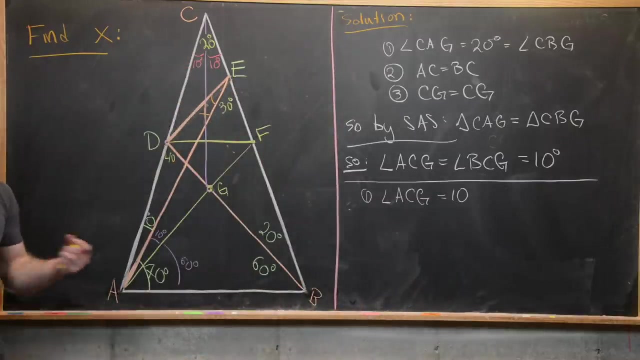 is also 10 degrees. So now we're going to make another SAS argument for the congruence of two more triangles, And in this case we're going to notice that first of all we have the angle ACG, So that's equal to 10 degrees by just our recent calculation, And then it's given that the angle 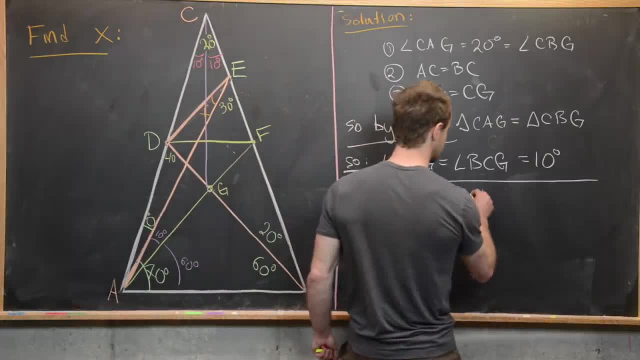 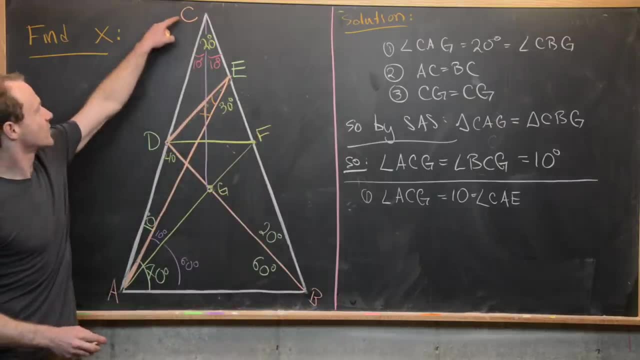 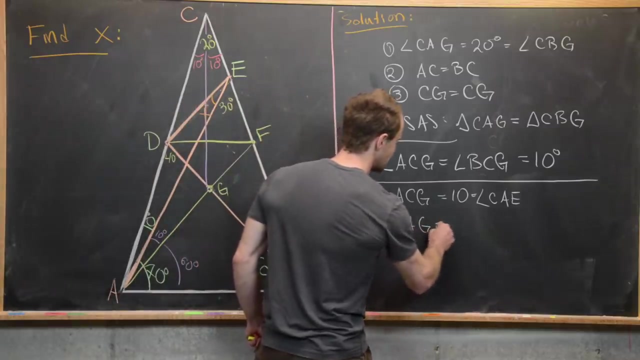 CE is also 10 degrees, So that was given at the beginning of the problem. So this is also equal to angle CAE. So both of those are equal to 10 degrees. And then, furthermore, we have angle CAG is 20 degrees, So let's write that down. So CAG is also 20 degrees And that's also equal to. 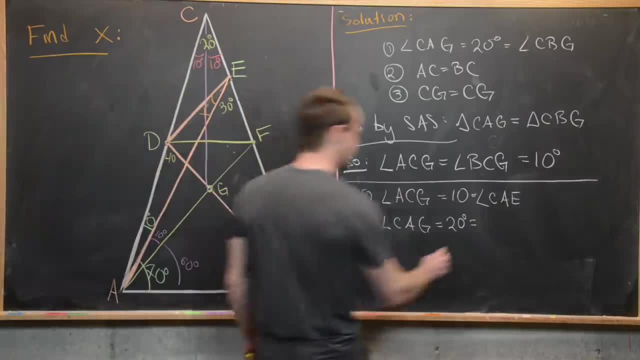 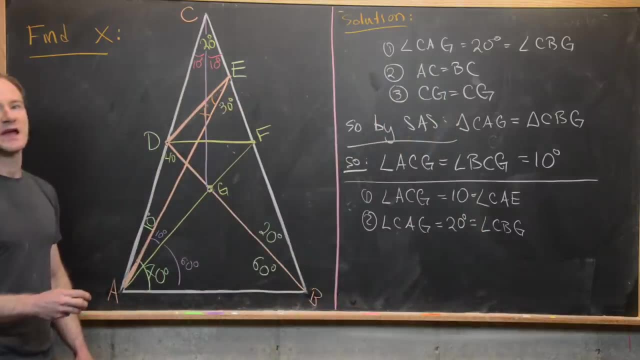 this angle CBG. So let's write that down as well. So CBG. So we've got two angles, two pairs of angles which are congruent, And now we can make a trivial equality of sides, And the two sides that will be equal are AC with itself. So in other words, AC with itself. And again, 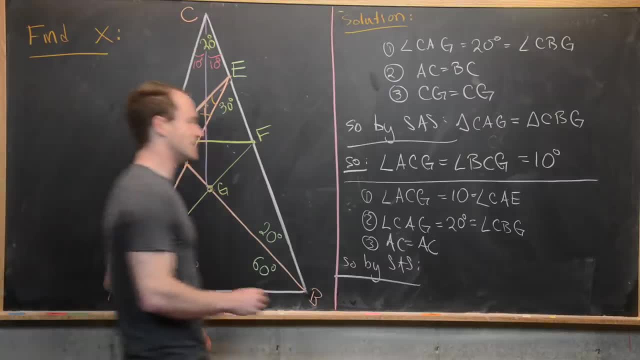 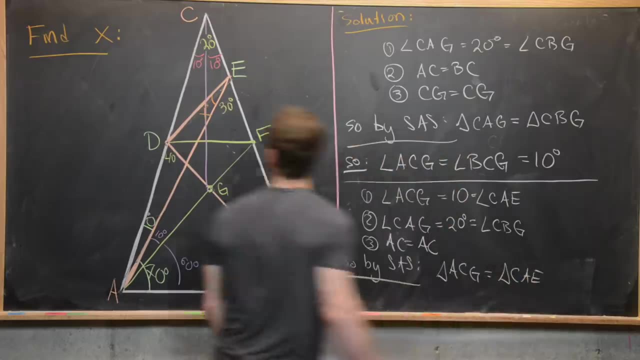 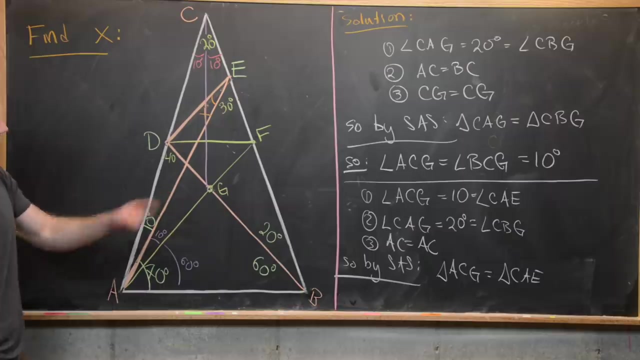 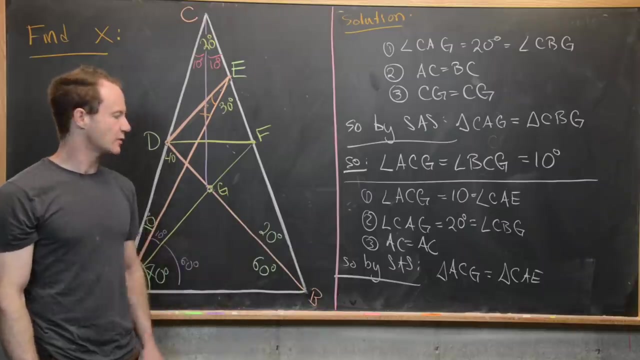 by side, angle side, we have the congruence of two triangles, And those two triangles are triangle ACG and triangle CAE. Okay, so let's look at that. So triangle ACG: So it's this one over here with triangle CAE, So let's look at that one. CA with E. Good, Okay, so now that we've established, 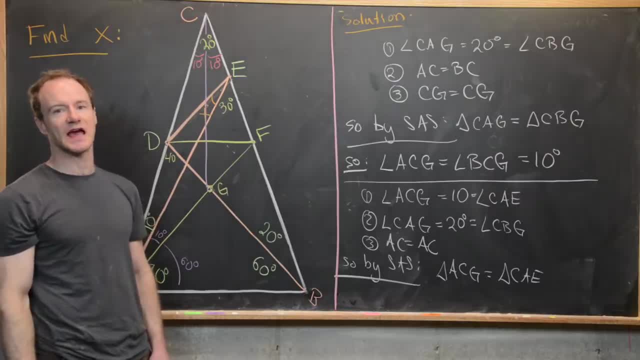 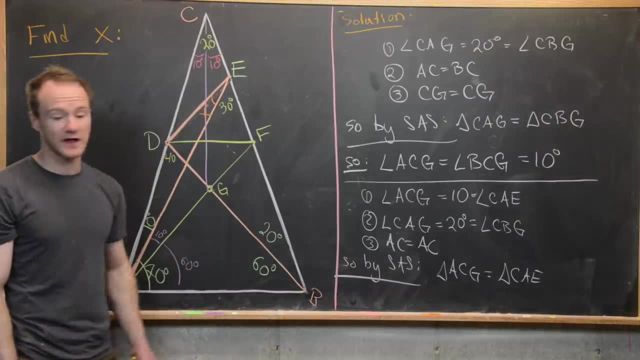 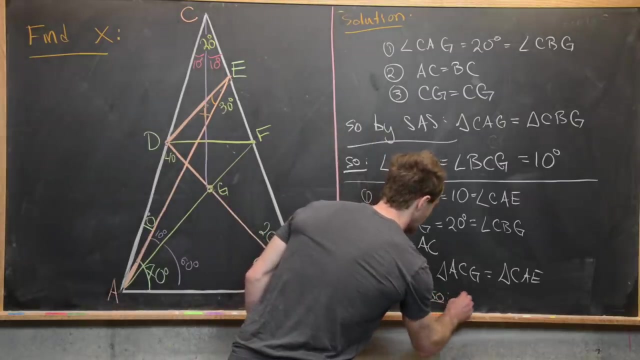 the congruence of triangle ACG with triangle CAE. we know that we have the congruence of the corresponding sides And the sides that will be important to know that are congruent for us are AG with CE. So let's notice that here we have side CE is congruent to side A. 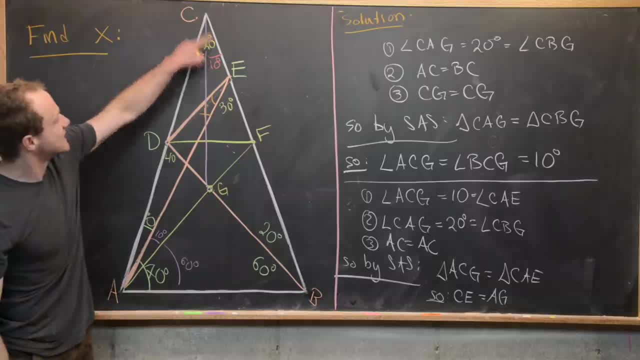 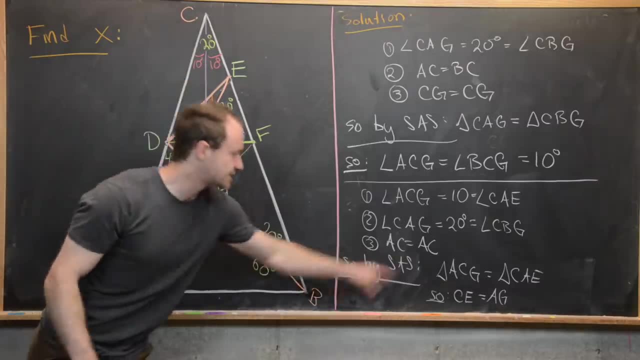 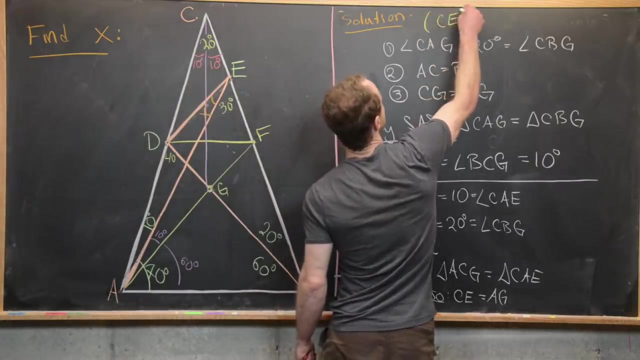 G. So let's just look at that real quick. So here we have CE and AG, So those are corresponding sides from the triangles that we have shown to be congruent. So that's actually really important. So let's go ahead and save that up here. We'll say that CE is congruent to AG. Okay, so the next. 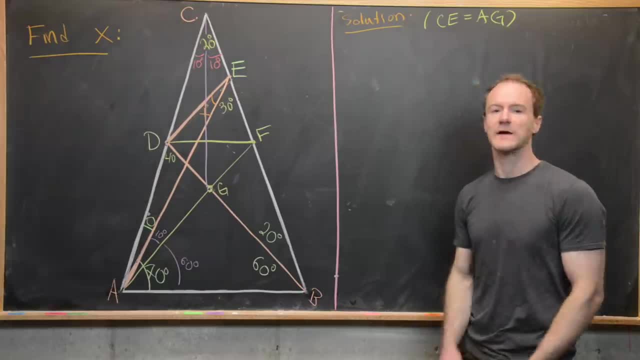 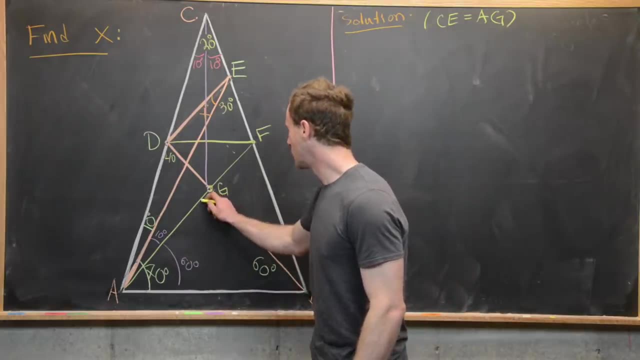 thing I'll do is clean up this and then we'll go on to the next step. Okay, so the next thing that we want to notice is that, since here we have a 60 degree angle, here we have a 60 degree angle. we know that this is also a 60 degree angle, But then it's easy to 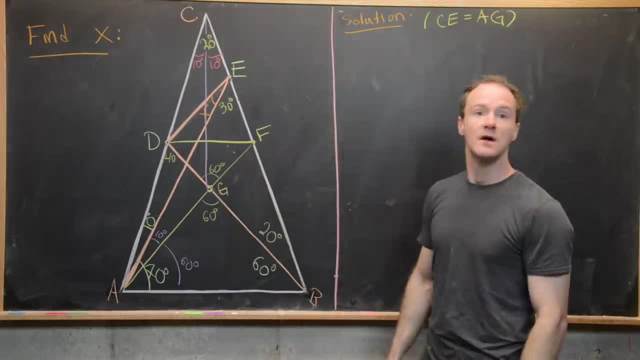 see that the opposite angle is also 60 degrees. But then we know triangle ADF and triangle BDF are congruent by an earlier calculation, which makes these two angles the same. But that's going to make those two angles equal to 60 degrees. But now we've got a triangle with three 60 degree. 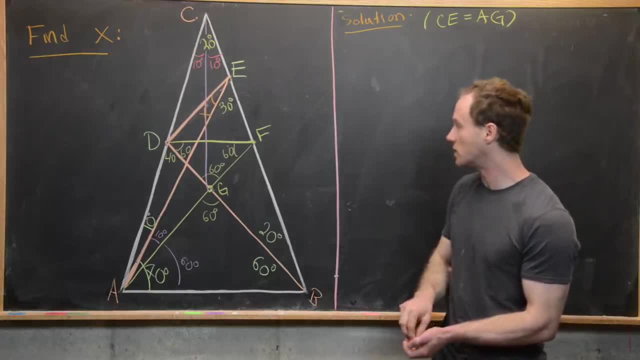 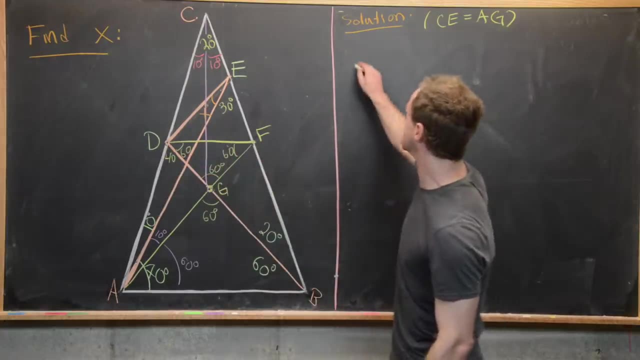 angles, which means that it's an angle that's congruent to the triangle BDF. So we're going to do an equilateral triangle which tells us that all three of these sides are the same. In other words, DG is the same as GF, which is the same as DF. So let's write that down real quick. So here, 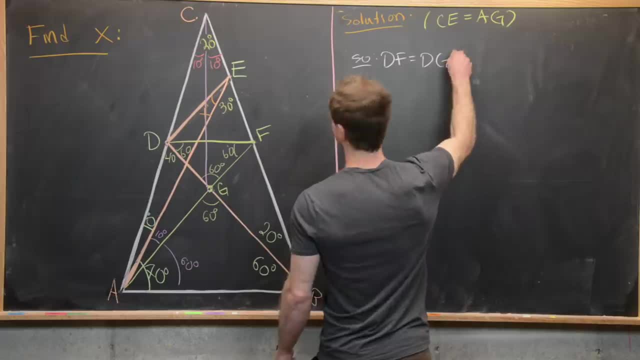 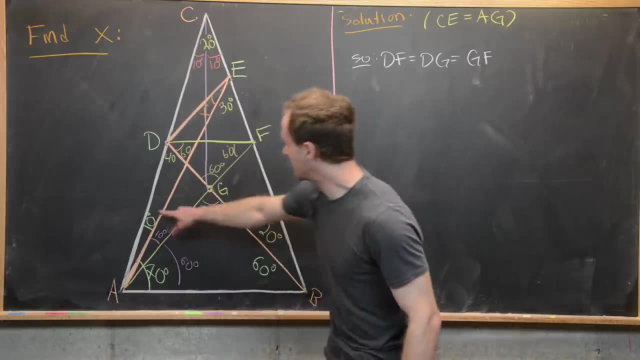 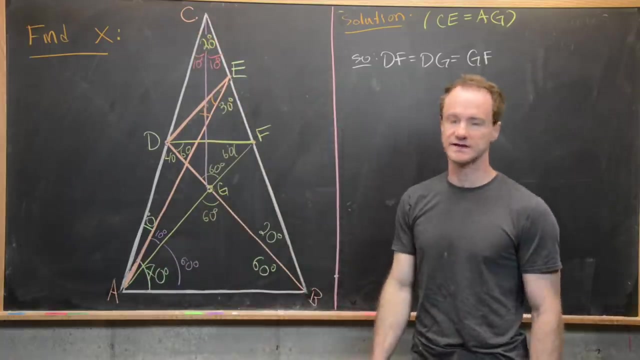 we have DF is congruent to DG, which is congruent to GF. Okay, the next thing we want to notice is that angle CAF is 10 plus 10 or 20 degrees And angle ACF is also 20 degrees, But that's. 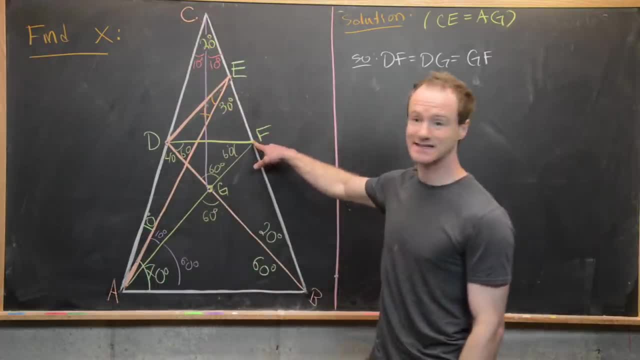 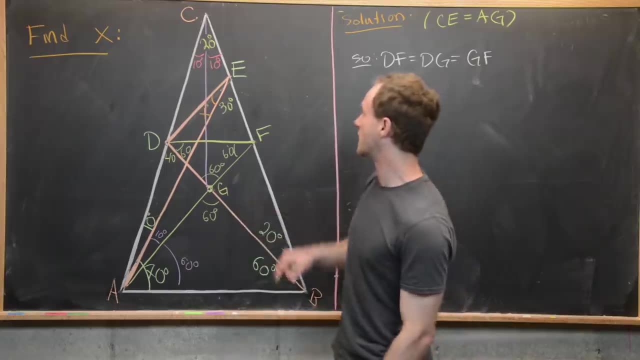 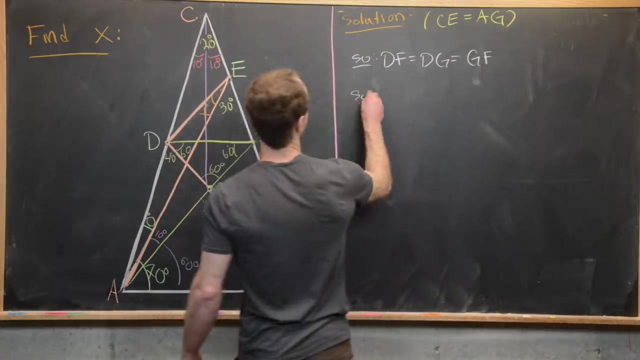 going to make triangle CAF an isosceles triangle, because we have two equal angles here, But that makes the opposite sides of those equal angles congruent. So in other words, we have this side CF is congruent to this side AF, And so let's just go ahead and write that down over here. So we have. 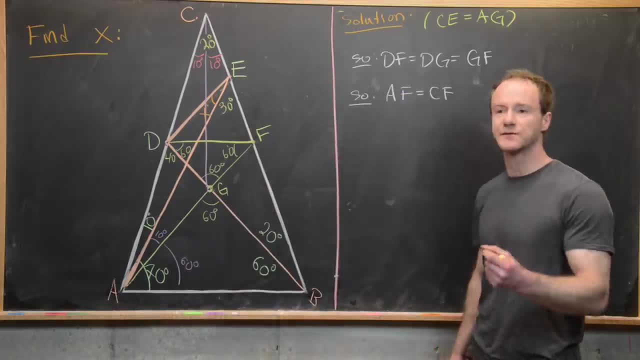 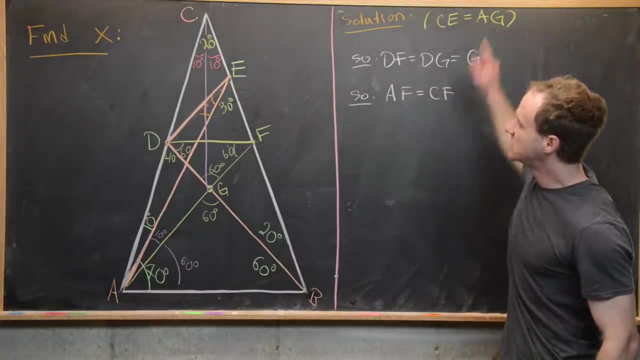 AF is congruent to CF. Okay, so from here we want to use the fact that AF equals CF and CE equals AG to notice that FG is the same thing as FE. So let's go ahead and look at that real quick. So CE. 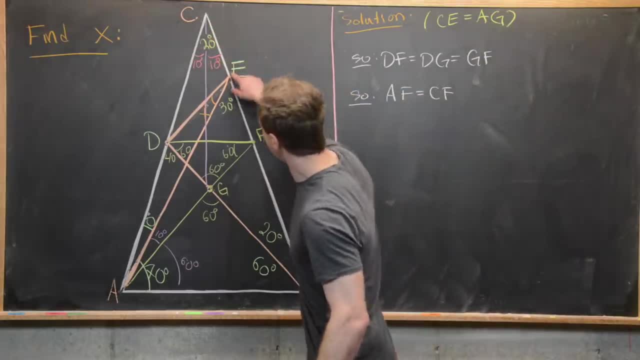 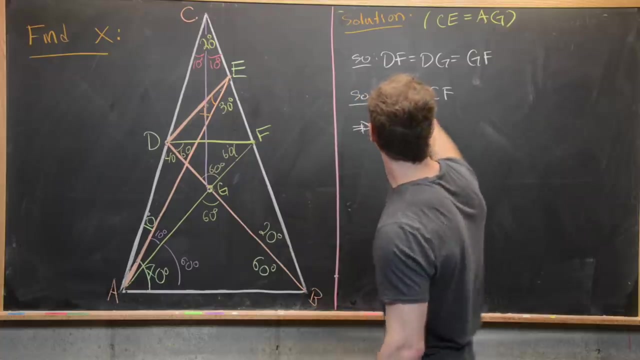 equals AG. So that would be this line segment here and this line segment here. Okay, good, But then we also know that AF is equal to CF, but that makes the remaining pieces congruent. So, in other words, from this fact right here and this fact right here, we see that FG is congruent to CF. 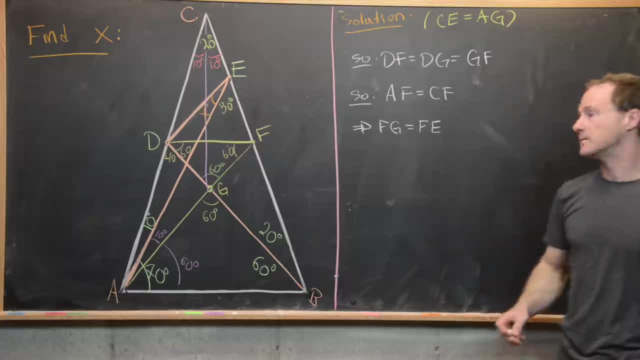 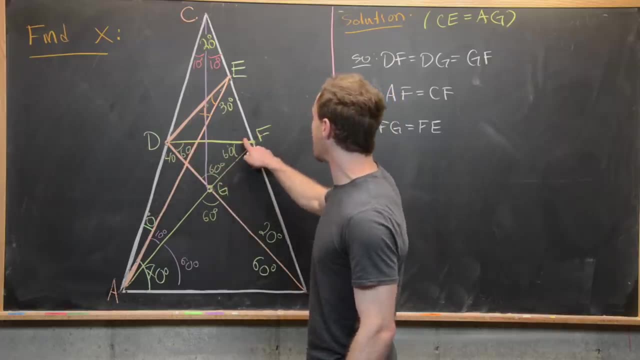 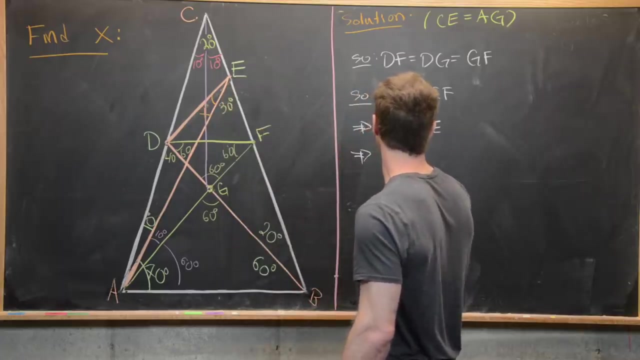 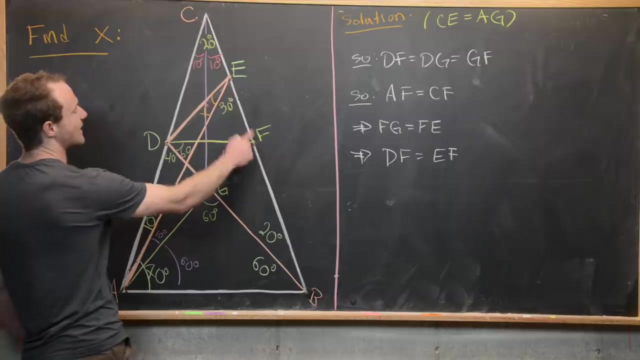 Okay, great. But then we know that this is an equilateral triangle, which means that FG is congruent to DF, but that means that DF is congruent to EF. So let's go ahead and write that down. So DF is congruent to EF, But that makes this triangle- right here, DFE, an isosceles triangle with equal. 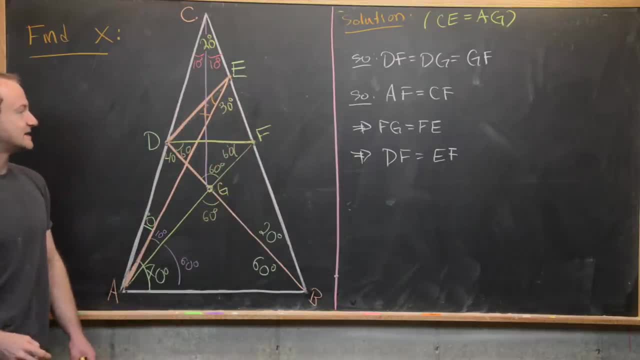 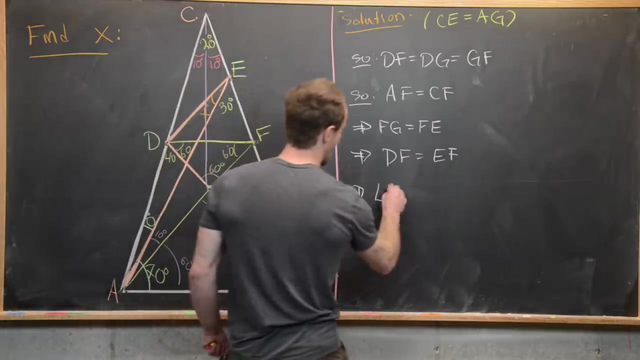 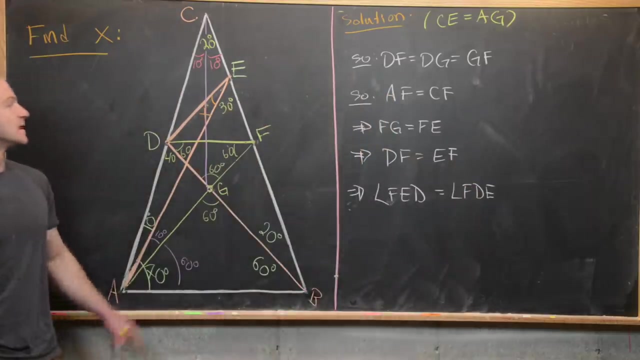 sides DF and EF. But that means the angles opposite those sides are also equal. So notice, the angles opposite those sides are FDE and FED. So notice, that's going to tell us that angle FED is congruent to angle FDE. Okay, good, But now notice that angle FED and angle FDE are both equal to EF. So 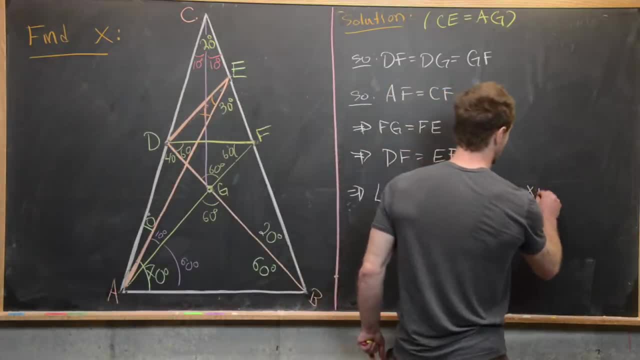 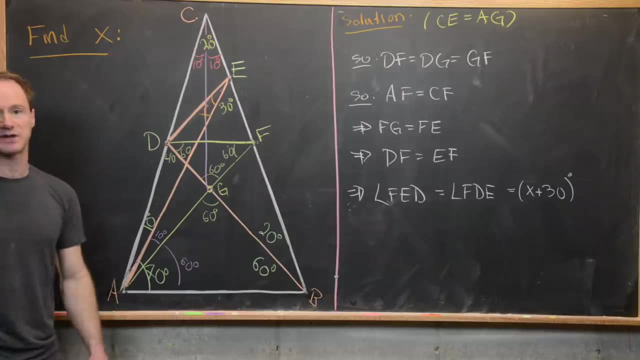 let's go ahead and write that here. These are both equal to X plus 30 degrees, And that's because they're congruent, And FED is X plus 30 degrees. So now the next thing that we can do is use the. 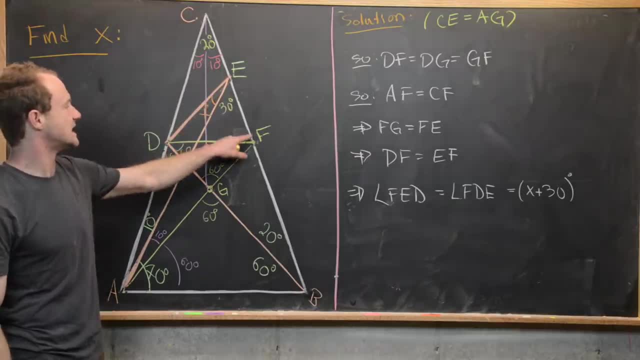 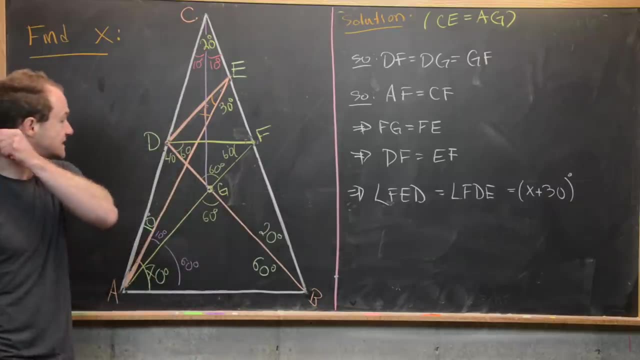 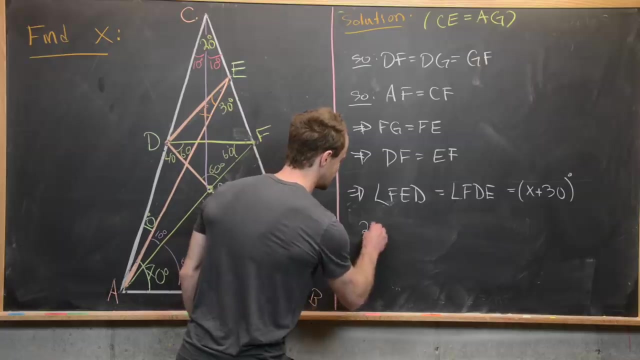 fact that the angle sum of the triangle DEF will be 180 degrees. Now two of those angles are congruent: angle FED and angle FDE, and they're both equal to X plus 30 degrees. So if we write those two together we'll get 2X plus 60 degrees, plus the remaining angle, which is DFE. So let's 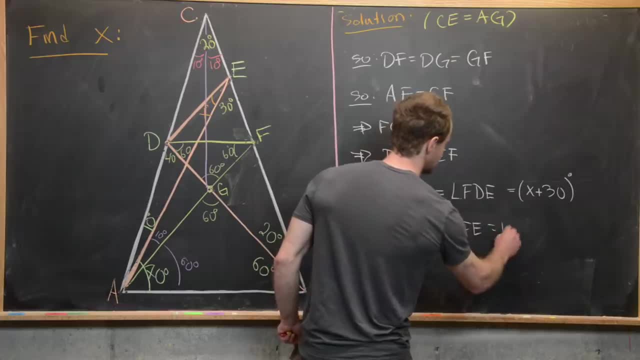 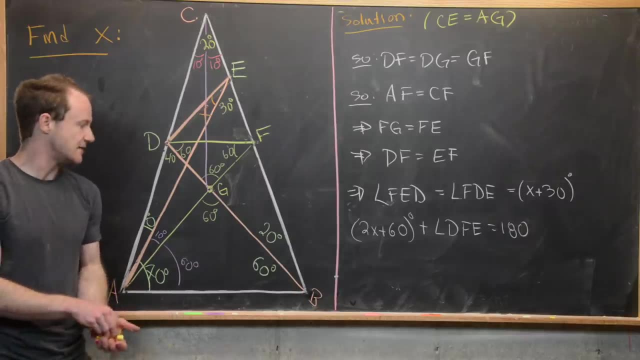 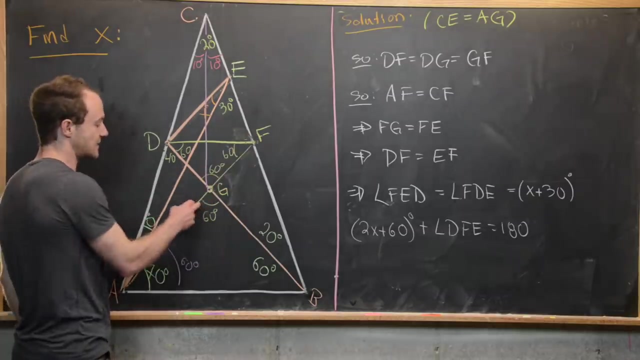 put that down, angle measure DFE. that needs to be equal to 180 degrees. But luckily we can calculate angle measure DFE pretty easily And we can do that in the following way: So we know that here we have a straight line AF, but that's going to make the remaining part of this angle. 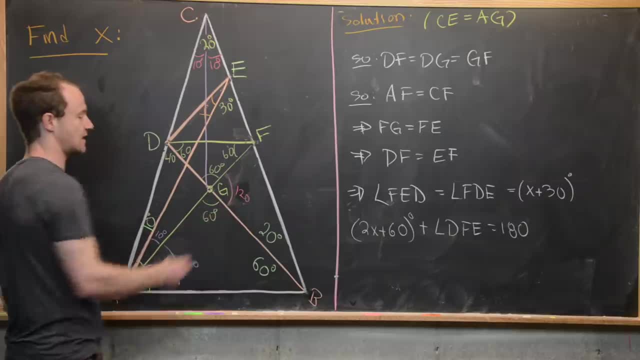 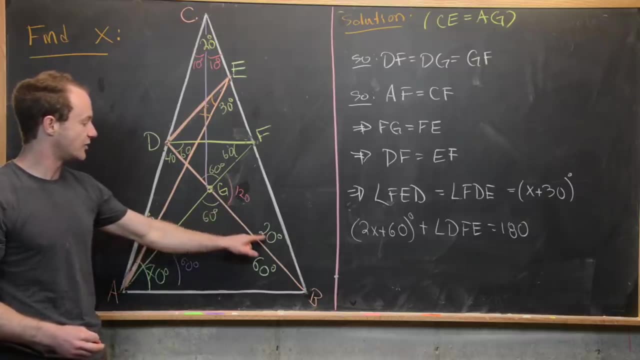 120 degrees, because that sum needs to be 180. And then, furthermore, because the angle sum of a triangle is 180, we have 140 from these two angles. that's going to make this 40. And then again, because this is a straight line, we know that this entire angle measure is 180. But here, 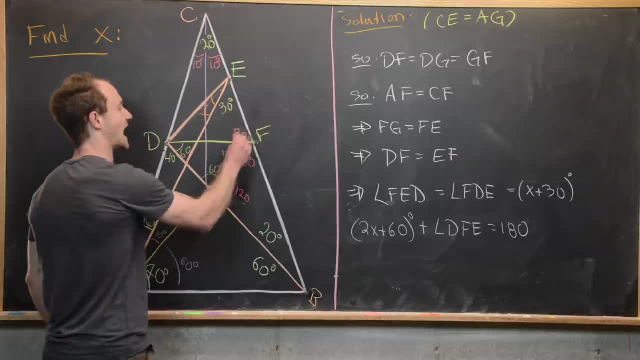 we have 60 plus 40 is 100. So what's left over here is 80.. So, in other words, angle measure DFE is 80 degrees. So we know that this entire angle measure is 180.. So we know that this entire angle. 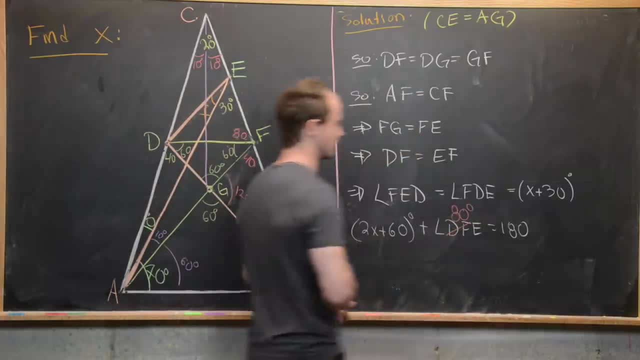 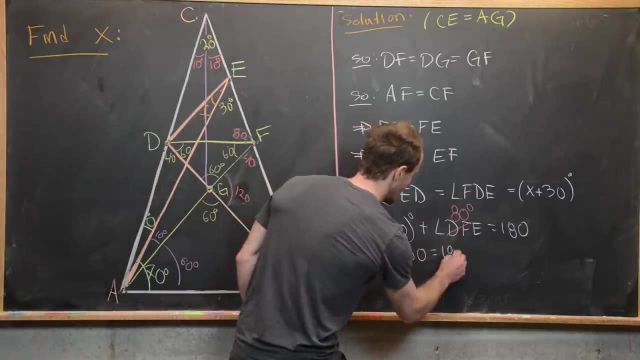 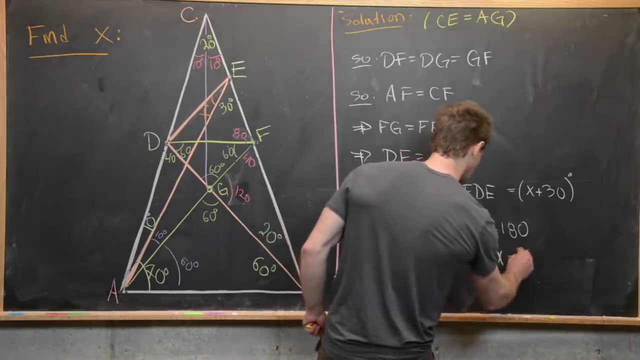 measure is 180 degrees. So we have this: here is 80 degrees, But then that's going to tell us that 2X plus 60 equals 100 after subtracting the 80 over. But that's going to tell us that 2X equals.